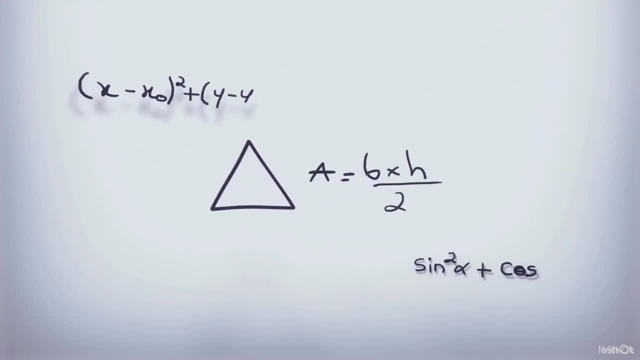 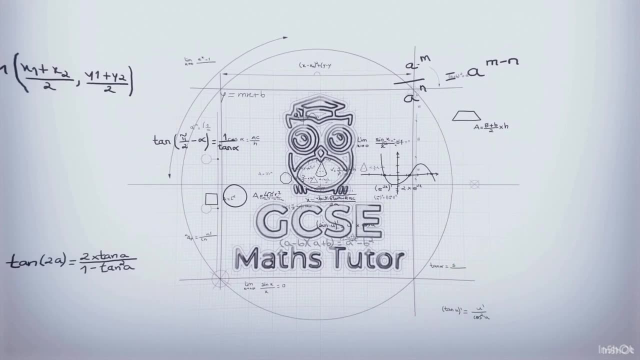 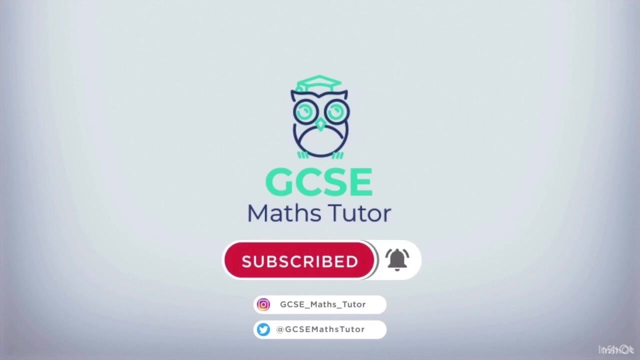 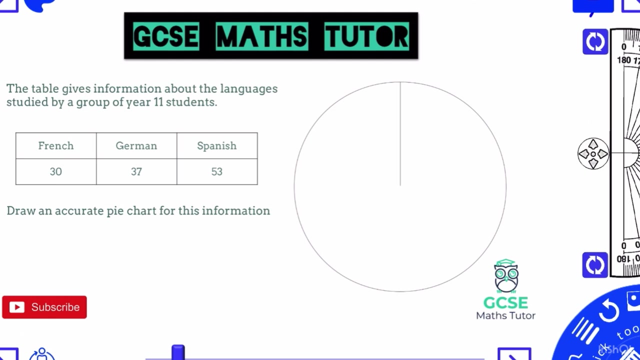 Okay, so in this video we're going to have a look at pie charts. Now, the great thing about a pie chart- and we are going to be looking at this in a non-calculator method, but the great thing about a pie chart- is that all of the numbers in the question that we're 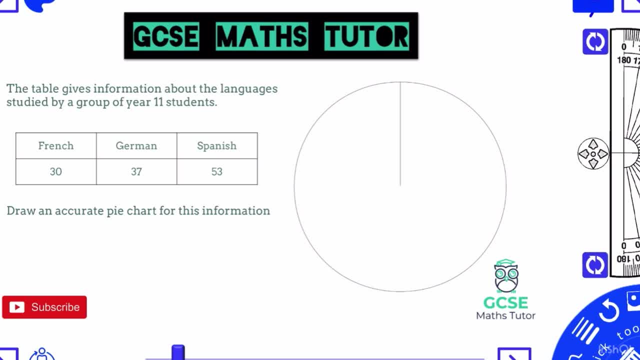 going to have a look at need to add up to 360. We know that around a point in a circle all the angles add up to 360, so that in order for our pie chart to work, it has to add up to that number. So if we look at our question, we're going to find the numbers that are associated. 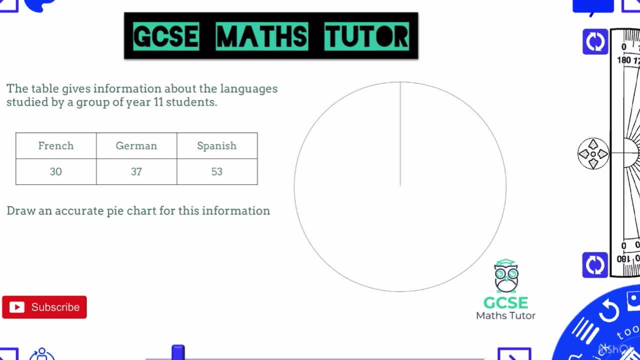 with our question, we're going to get the numbers to add up to 360, and then we're going to draw it using our protractor, So we're going to run through all of that. so I've got a question for you to practice and one final question for us to have a look at. but 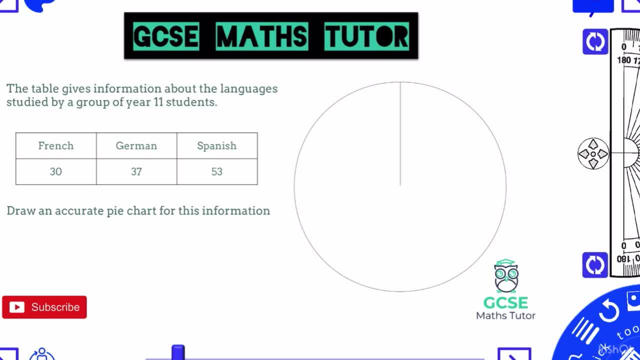 relatively quick video looking at drawing pie charts. So this question here says the table gives information about the languages studied by a group of year 11 students and it says that 30 study French, 37 study German and 53 study Spanish. and it says draw an. 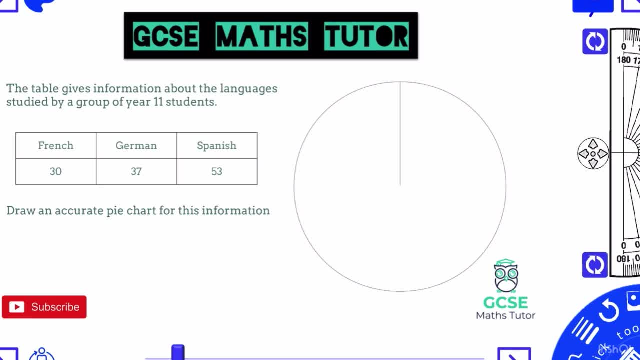 accurate pie chart for this information. So the first thing we want to do is add up all these numbers. So if we add up 30,, 37, and 53, let's have a look- that adds up to 120.. Now we know what the total is, and the total there is 120.. So in order to get this to 360,. 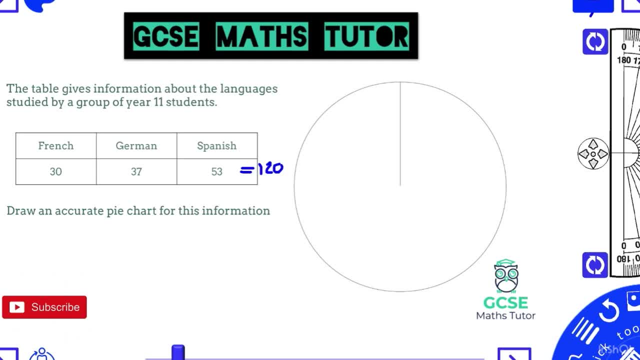 either you just have to think about that in your head. what do you multiply 120 by to get to 360, or we could just do 360 and divide that by the total there, which is 120.. So 360 divided by 120 is 3, meaning that we're going to have to multiply all of these by. 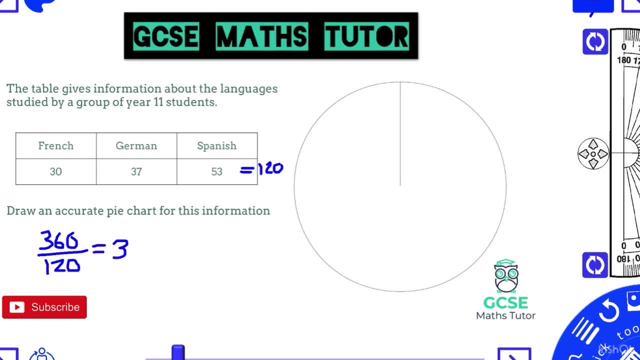 3 to get the angle in each portion of the pie chart. So if we multiply them all by 3, we'll just write times 3 next to them all. There we go: times 3, times 3, times 3.. That 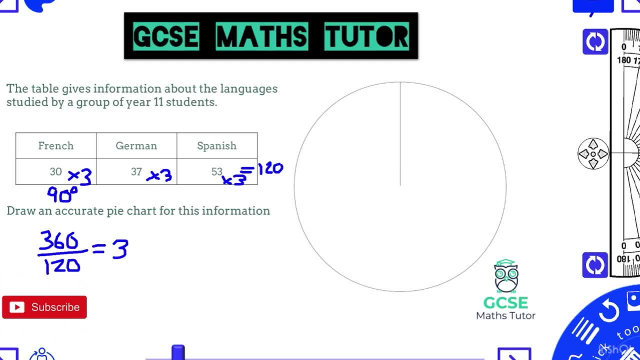 would mean that 30 would become 90 degrees, and these are our angles. now We would have 37 times 3,, which would be 111, so that would be 111 degrees, which is a bit of an awkward one to draw, and 53 times 3 would be 159.. So that is 159 degrees. Now, that is the main. 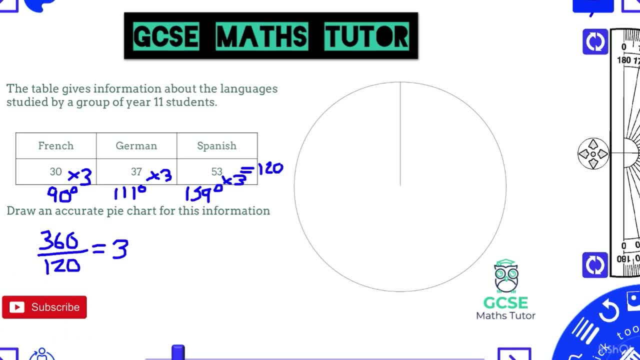 bit of our working out. now, We know all of the angles that we need to draw. we just actually need to draw them. So we're going to do that, So we're going to do that, So we're going to do that. So, when you've got your pie chart drawn like this, if it's given to you, if 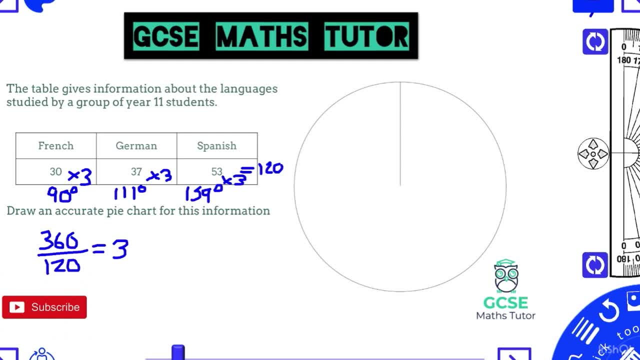 not. you're going to have to use a compass just to draw a circle. If you're making notes on this, I would definitely do that. Just get your compass, draw a nice circle. just make sure that you know where the centre of that circle is, so that you can draw this. 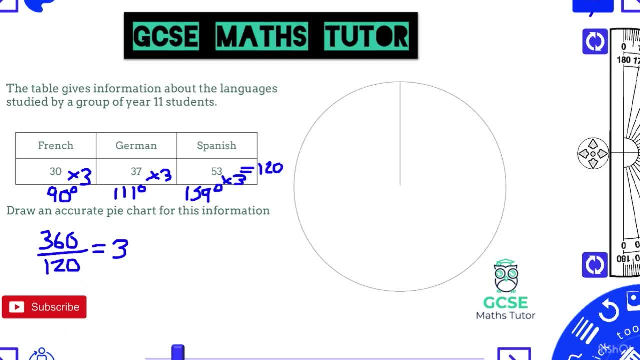 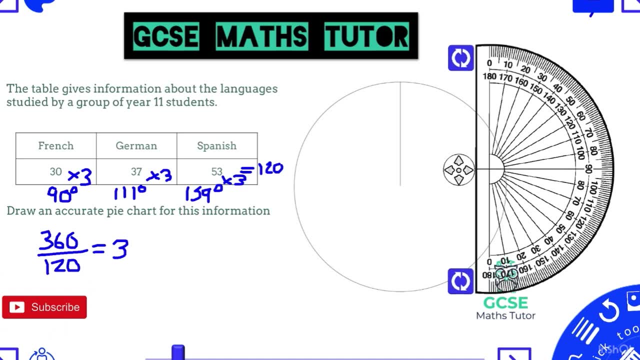 nice straight line going up, so you have a place to start from. So let's start with drawing on this French one, which is 90 degrees. We can put them all in at the same time, but let's do the first one. So get your protractor, pull it over the top of the pie chart, make. 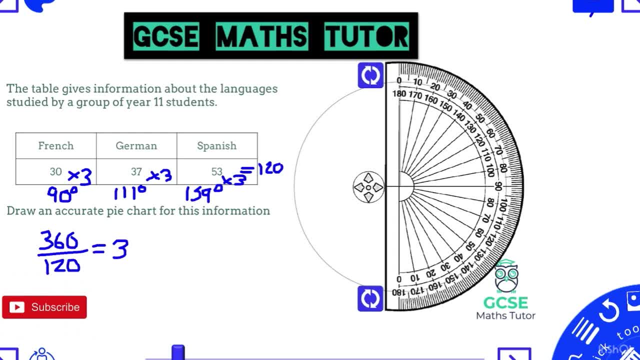 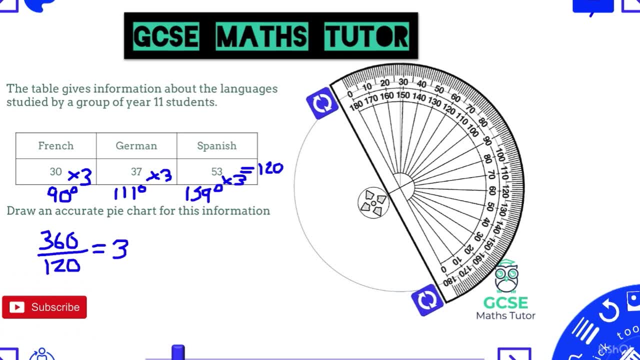 sure, that little crosshair in the middle of the pie chart is in the middle of the pie chart, is right on the centre. There we go, Just do that really nice and carefully. And then you also want to rotate your protractor so that the guideline where it starts at zero. 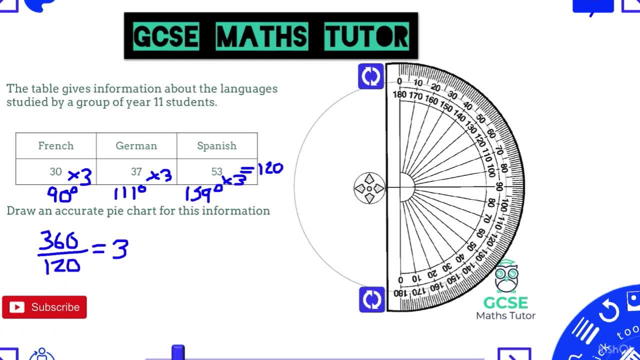 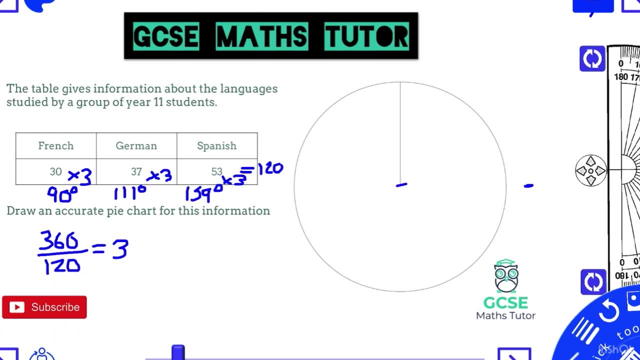 is lined up with the line that you're starting from, which is the one that's vertical. So there we go. That's nicely lined up. So I want to mark on 90 degrees. So I'm just going to mark the 90 degrees over there. There we go, Pull your protractor out of the way And 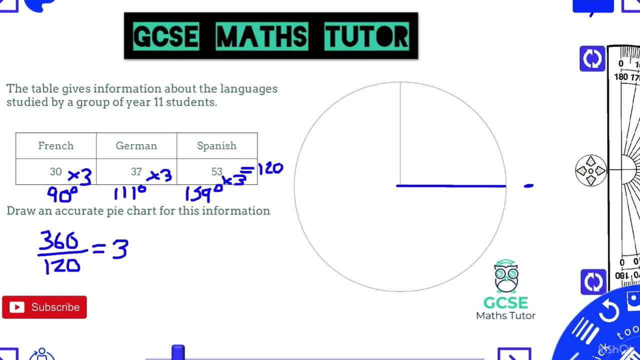 then you can obviously do it a little bit shorter, just to the edge of the pie chart. And there we go. That's your 90 degree angle. Now you can move on to the next one. But before you do, what I tend to do is I normally tend to label that section. So I'm just going to 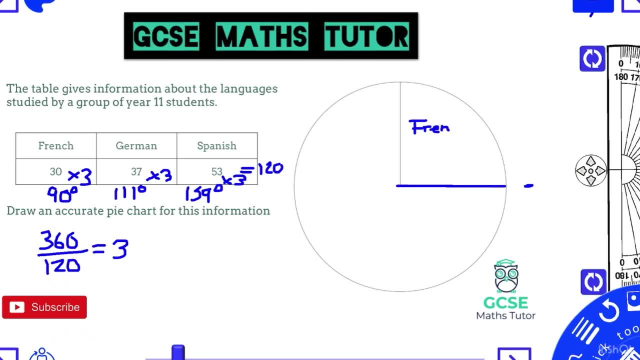 put French in there. So I'll put French in and I'll also put the degrees in there: 90 degrees. You could also put the 30 in there as well, but just to keep it a little bit simpler on the screen, it's going to leave it as French, with the 90 degrees. Okay, So? 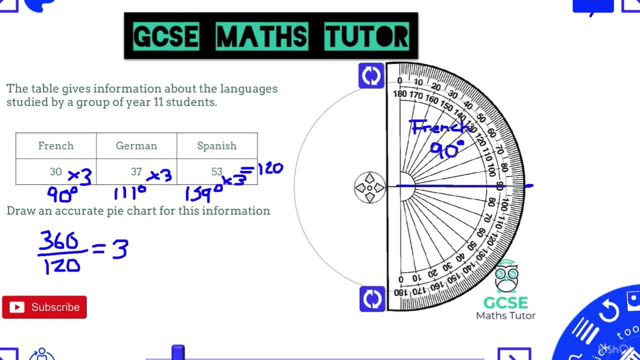 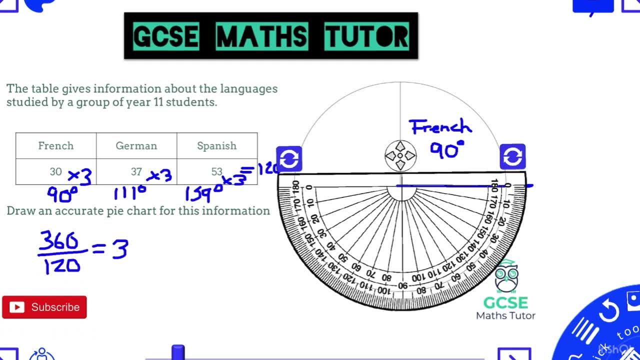 I'm going to move the protractor back onto the centre Now. we just want to rotate the protractor round so that the zero is lined up with our new line. So we can carry on from that point. And again I'm using the outside numbers, And now we need to do 111 degrees. 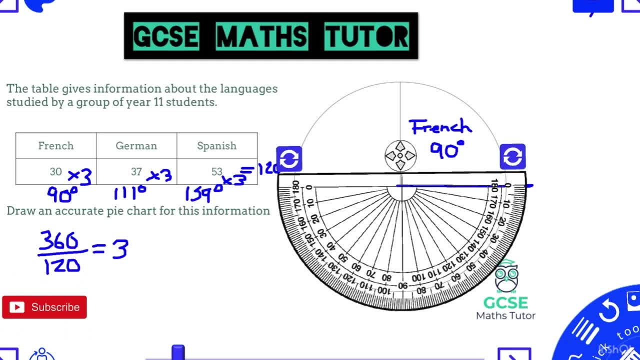 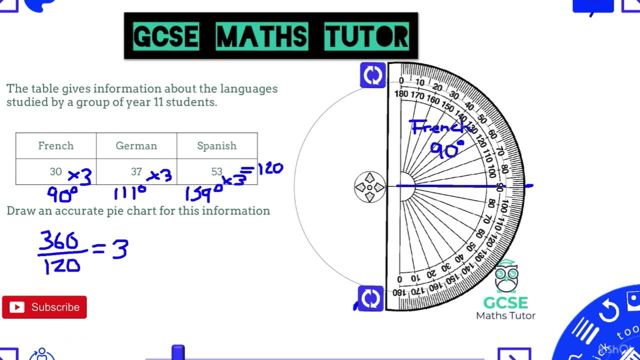 So, past the 90,, 110,, 111 is just past that And you're going to have to just get it as accurate as you can. There we go. There's 111 for me Again. just pull that protractor out of the way and we can draw in a nice straight line again from the centre. So from the centre. 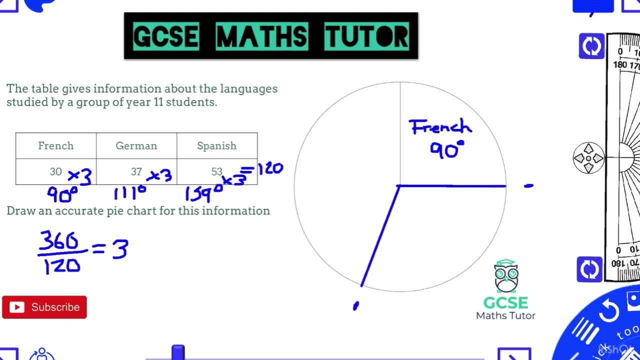 a pencil, join it up. I'm just going to shorten it a little bit. There we go. You can do that a little bit easier when it's not on a screen, but there we go, Using your ruler and a pencil. I'm just going to label that So that would be German And that was 111 degrees There. 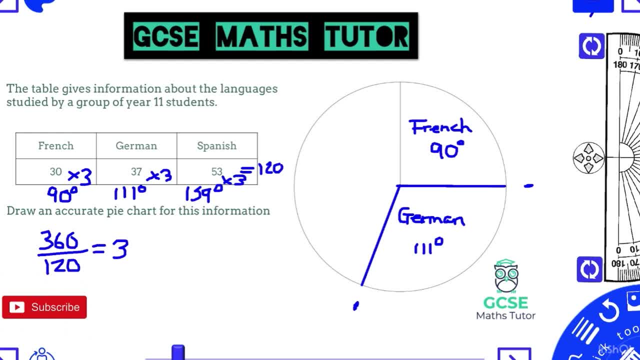 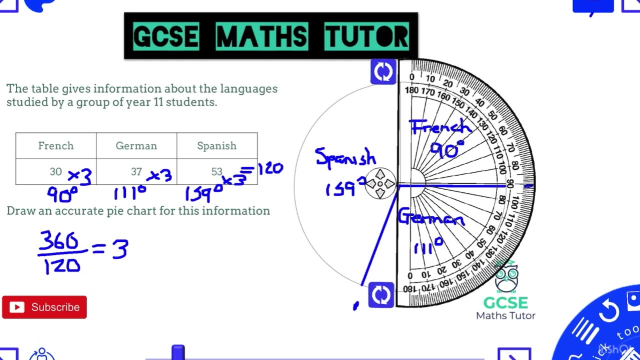 we go And the last part of the pie chart here, which, as we only have one left, is Spanish, So we'll label that as Spanish And that is 159.. A good bit of practice here that you should do is you should stick your protractor on. 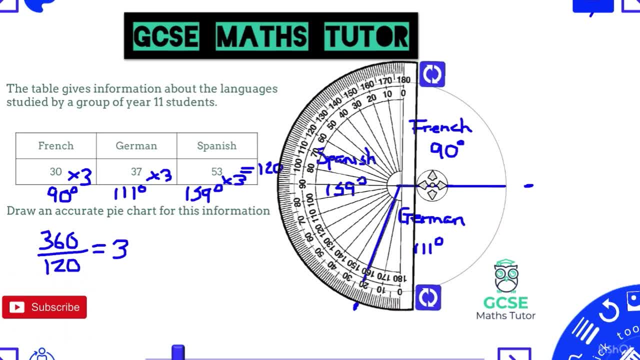 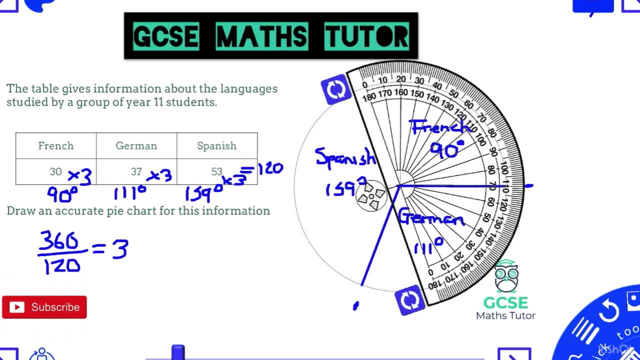 Just measure that final angle there. So I'm going to flip it around the other way, Measure to see if that's 159.. It might be a little difficult for you to see on the screen there, but that comes out as around 159 for me. So I'm happy with that. It's an accurate pie. 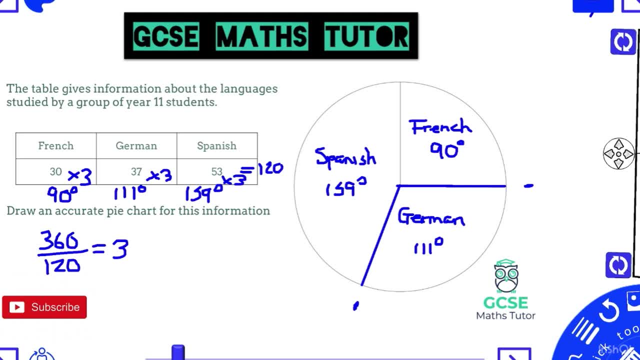 chart. All of the angles match up to what I wanted them to. And there we go. There's your pie chart. Okay, So that's how you go about drawing it. That's how you get the angles. Remember, they've got to add up to 360.. So that bit of working out there, where I added 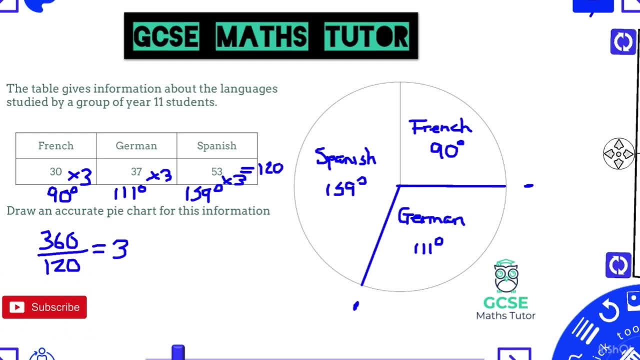 a total and did 360 divided by that total, allowed me to see what I needed to multiply all those numbers by so that they all added up. And another good bit of practice that you could do is take those three numbers and just add them up And you can actually see. 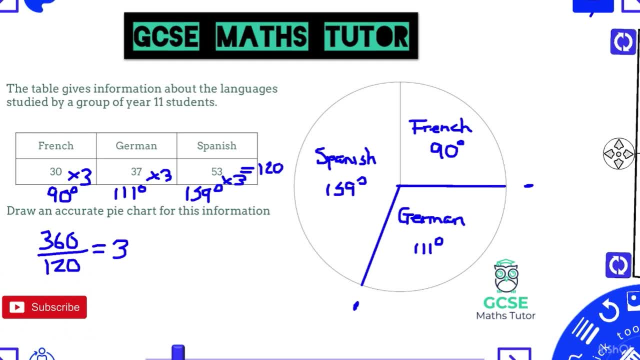 159, 111 and 90 do all add up to 360.. So we've definitely got it right, Okay, So there we go. That's how you're going to do it. I've got one for you to have a go at, So let's. 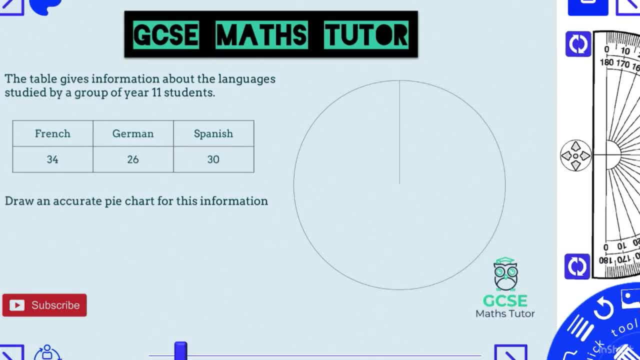 have a look at that one now. Okay, So here's your question. So if you are comfortable drawing a pie chart and using a protractor, then what would you do? Well, if you're comfortable drawing a pie chart and using a protractor, then what would you do? Well, if you're comfortable. 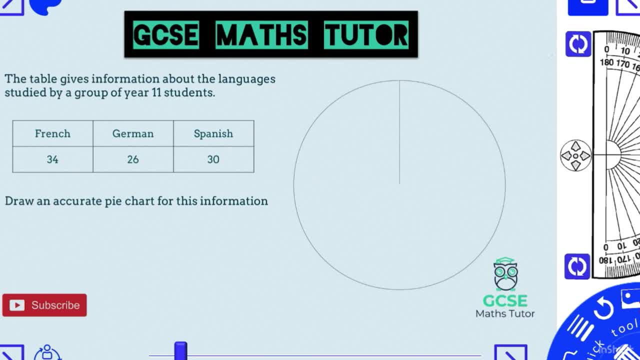 drawing a pie chart and using a protractor, then what would you do? Well, if you're comfortable, really, all you need to practice here is just getting those correct angles, Although, if you have got a compass with you and you can draw a circle and you've got your protractor. 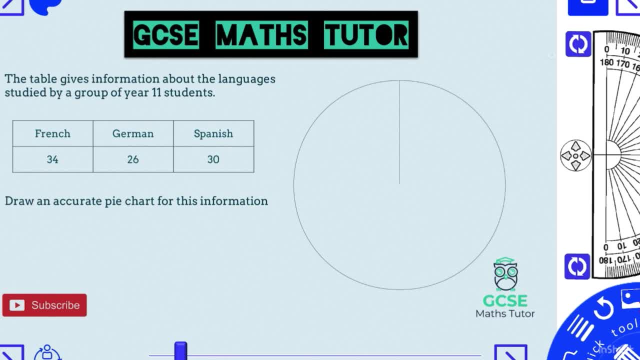 on you, then do feel free to have a go at drawing the pie chart as well, But otherwise pause the video there. have a go at this one and we'll go over the answer in a sec. Okay, So let's have a look then. So for this one here, we just need to add up what we've got. 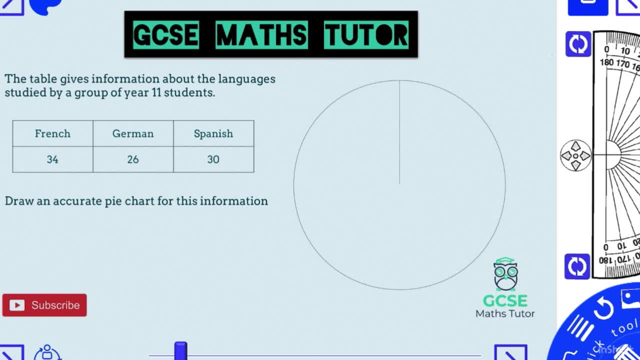 So 30,, 34 and 26. Now they add up to 90. So at the moment we've got a total of 90. Now what do we need to multiply those by? Well, we can work that out by doing 360 divided. 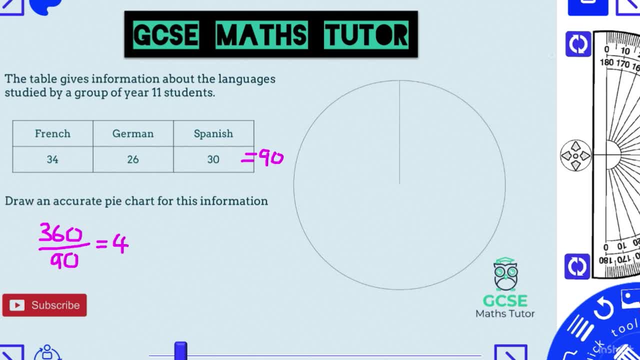 by 90, which comes out as four. So we need to multiply them all by four. So again, if I'm just going to put times four next to all of these, just to remind myself to multiply them all times four times, four times four, So 34 times by four, Let's just work that. 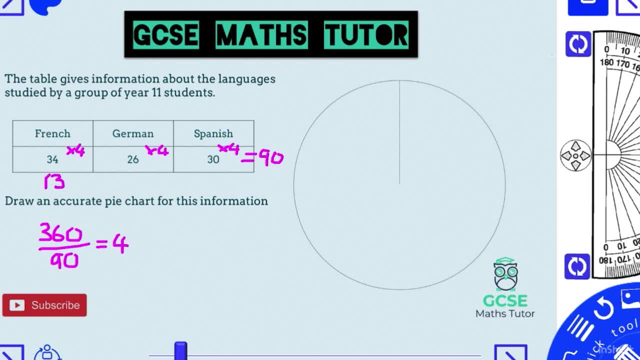 out on a calculator, just to speed this up: 136, 26 times four. Obviously, just take your time with these- 104 and 36.. 30 times four is 120.. Right, there we go. So there's our three angles. So if you've got those, 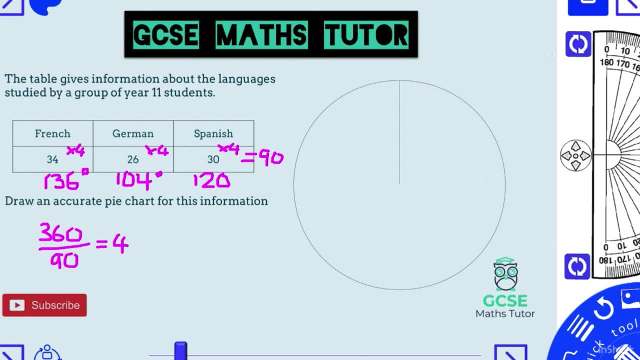 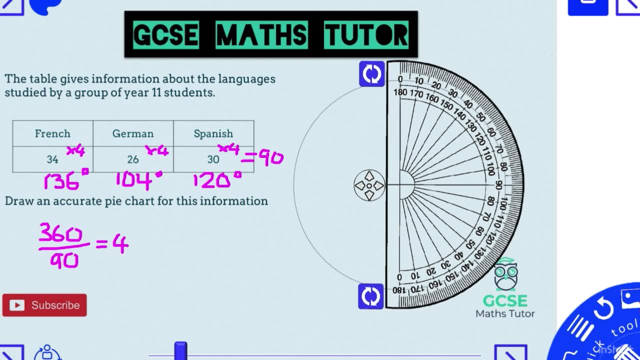 angles, then you should be pretty well set for drawing pie charts now. But let's just plot that or draw that onto our pie chart. So line it up with the center, go to 136 degrees, So 90 on the outside, 110,, 120,, 130, and just a little bit past the five, 136, just there. There we go. Join that up. 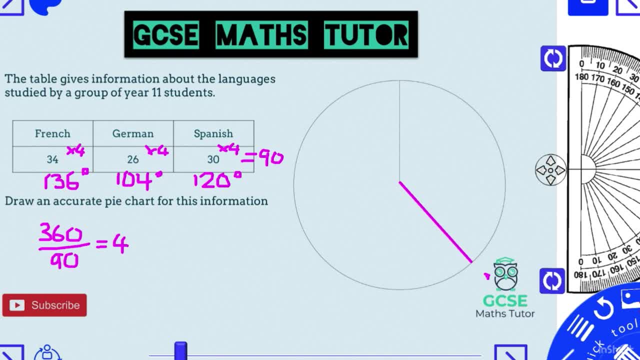 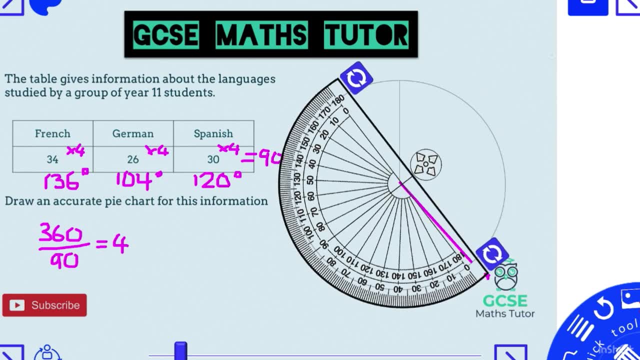 with a nice straight line, I'll label that in a second. So that's our three angles. So if you've got that in a second, And then back to the center And we need to measure out the 104 degrees, So I'll 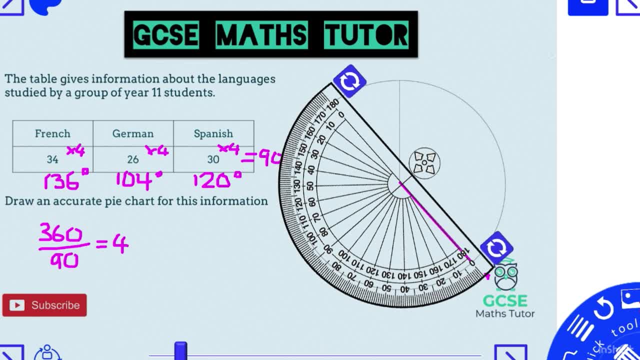 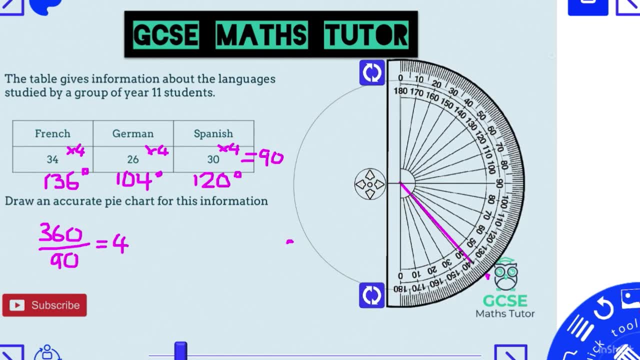 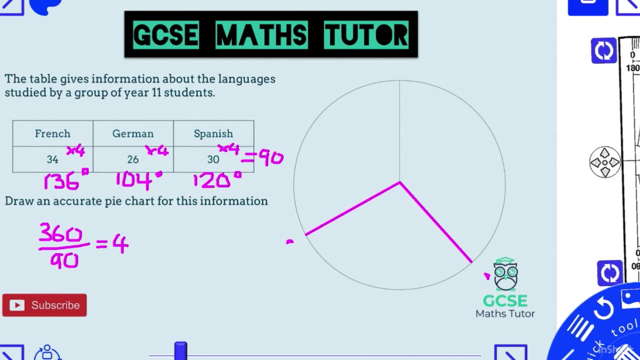 line that up with my pink line And we want 104 degrees, So past the 90,, 104, just there. And there we go. We'll join that last line up And there we go. And then, obviously, just not forgetting to, 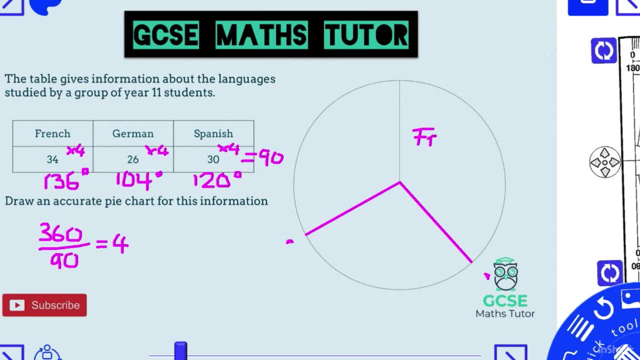 label them all. So you've got French, There we go. We have got 136 degrees in there. We had German, There we go With 104 degrees, And also Spanish with 120 degrees- There we go, Right. So there we go. There's your pie chart. Well, 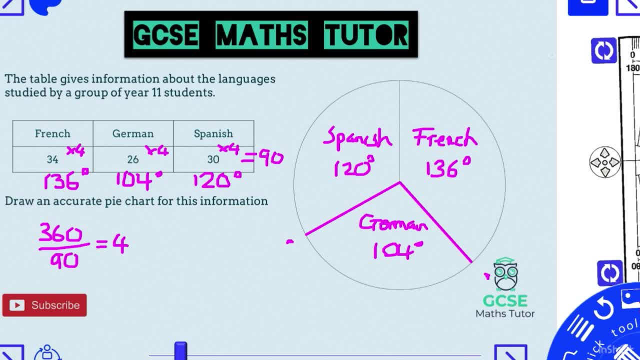 for actually drawing them, But there is another question that you could be asked, So we're going to have a look at one more question. That is going to be our last one before we finish, so we just need to discuss that and that will be the end of 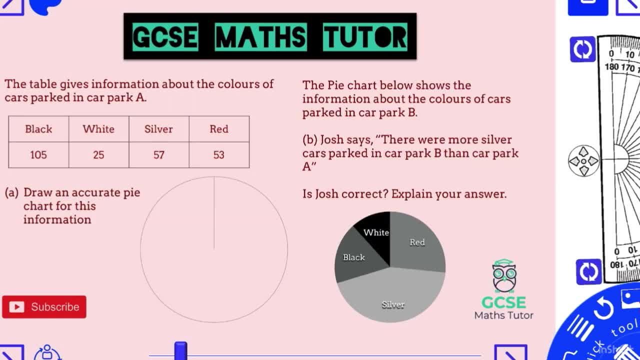 pie charts. So let's have a look at that one now. Okay, so let's have a read through this question. It says: the table gives the information about the colours of cars parked in car park A, and then we've got four different colours for different cars there and it says: draw an accurate pie chart for. 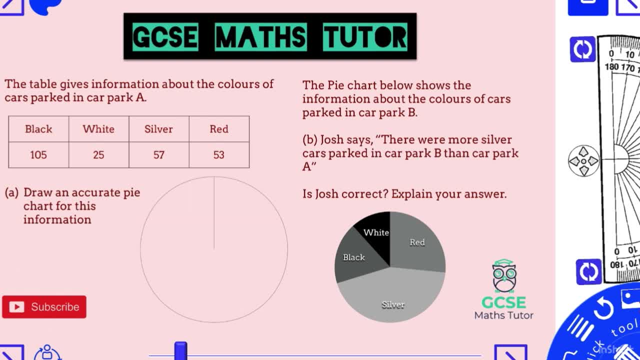 this information. It then says: the pie chart below shows the information about the colours of cars parked in car park B. Josh says there were more silver cars parked in car park B than car park A, and is Josh correct? Explain your answer. Well, we actually need to go about drawing our pie chart. 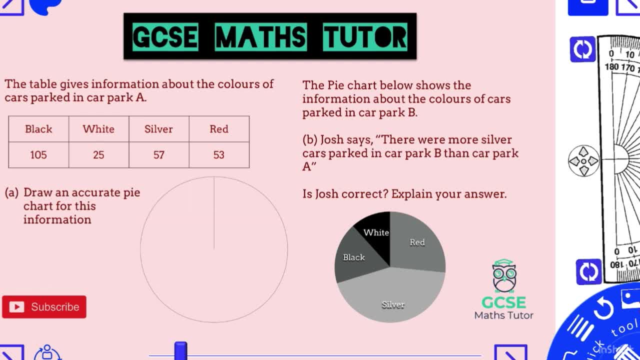 first. So if we draw our pie chart on the left, then can we- and here's the question- can we make a comparison between the two? Can we compare those two silver sections? That's what we're going to have a look towards in this question. So feel free to have a go at this question and pause it. Have a. 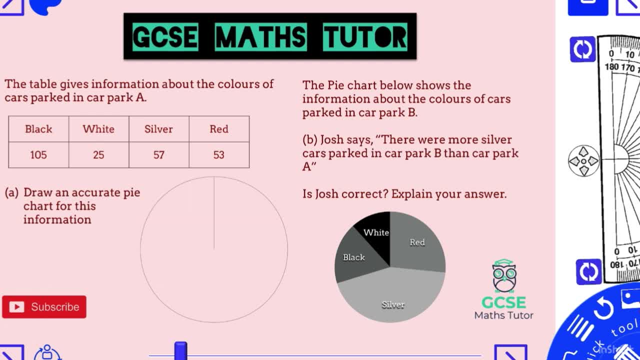 go at thinking about whether we can actually make that comparison with the pie charts And we will go over the answer in just a second, Right, okay? so if we go about drawing this, then Now at the moment this is quite a tricky one, because if you add all of those up, they add up. 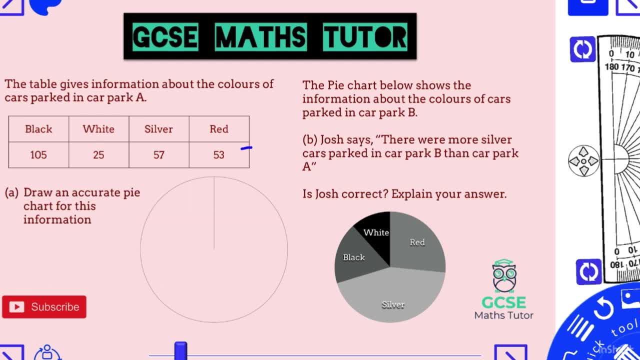 to 240.. So if they add up to 240, that would be quite a nasty one to do without a calculator. So if you were to do 360 divided by 240, what do you actually get as your answer? Because that's not a very nice one to do without a calculator. So how would we approach that? 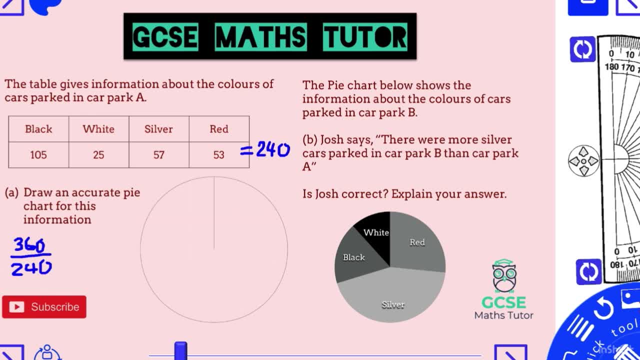 Well, I would say the best way to approach that would be to simplify the fraction. if you didn't have a calculator, Obviously, if you do, then that's nice and simple, You can just type it into your calculator. But if we simplify this, we get 36 over 24.. And then, simplifying that again, maybe we could. 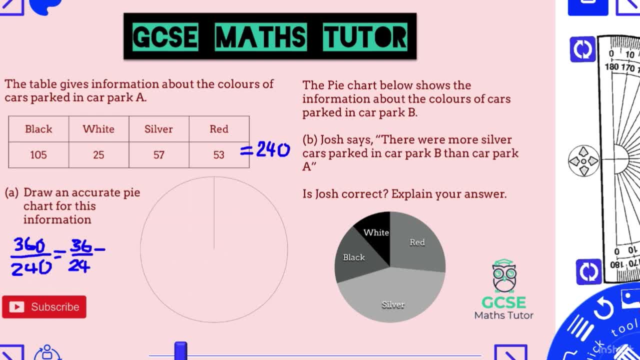 divide the top and bottom by 6.. Again you might spot bigger numbers that go in. but let's just simplify it So that would become 6 over 4. And then maybe we could do the same thing with the top and bottom. Maybe you could divide the top and bottom by 2. Which would be 3 over 2.. 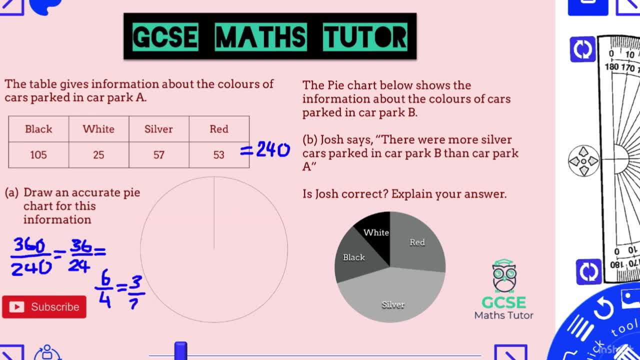 Right, so were getting there, And three over two is one and a half, So there we go. this means we actually have to times all of these numbers by 1.5, which isn't very nice. So we're going to times these by 1.5.. So multiplying them by 1.5.. Again, not very nice without a calculator. There we go. So if we times them by 1.5.. Now, that's not very nice, Etc. Okay, I'm going to podría actually write the little dot in there. So if we times them by 1.5.. So it's a fun, guys, a nice. 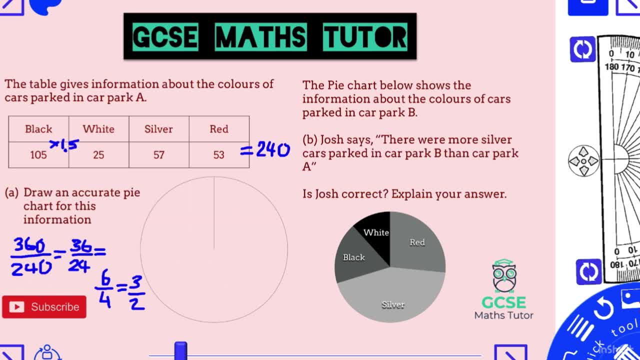 expression theory. but so let's just try again with that And we can actually do number sizes, and that's not very nice at all, because 105 times 1.5 is going to come out as a decimal. so if we're going to do that, then we get the answer. and again you can work this out doing some multiplication. 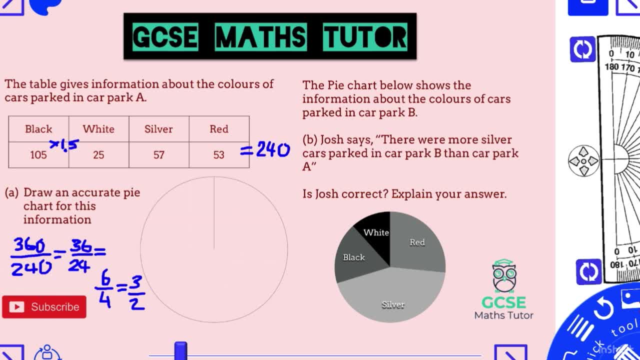 remember, when you times by 1.5, you can just halve it and add the half on. so half of 105 is 52.5 and if you add that on you get 157.5 degrees. okay, we'll have a look at that in a sec. the next one. 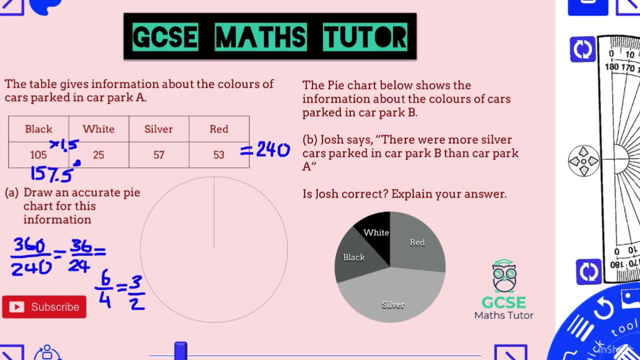 we've got 25. half of 25 is 12.5. add it on is 37.5 degrees. not very nice. again, I see these are all odd numbers, so it's going to happen for all of them. half of 57 and add it on again. you can take. 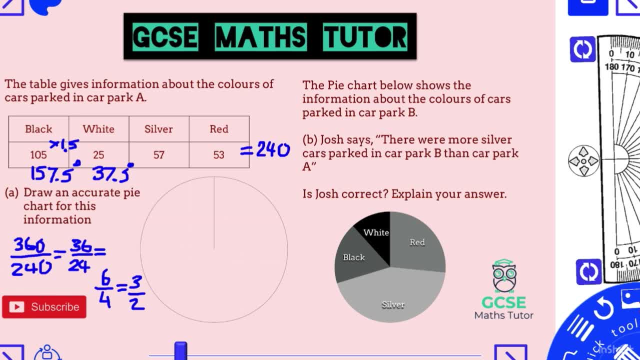 your time just multiplying this out using your normal method for multiplying decimals, though, and that comes out as 85.5 degrees, and the last one there is 53, so 53 times 1.5- again- let's take your time with that- comes out as 79.5 degrees. there we go right, so they've all come. 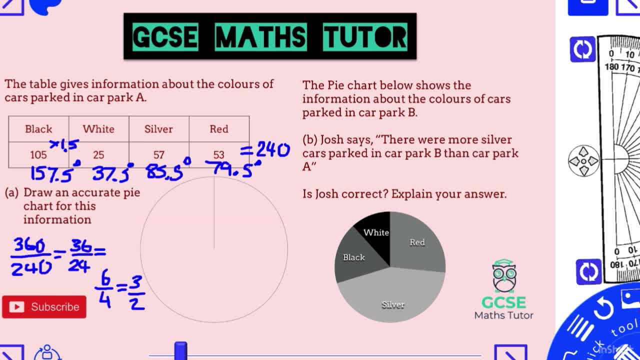 out as a 0.5. now that's not too bad. we can try and do this as best as we can. again, it says: draw it as you know, draw an accurate pie chart. but we can only draw it as accurate as we can. and there is. 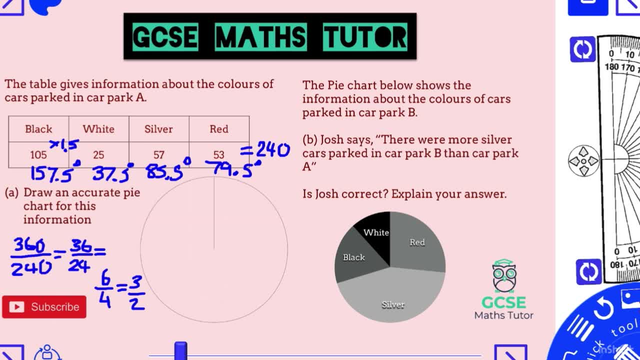 about a one to two degree allowance either side on the exam, because obviously some of these are quite difficult to plot, particularly this one where there's a 0.5. now what we could do is: you could, you could, you could round some of them up, some of them down, but then it's not going to be quite as 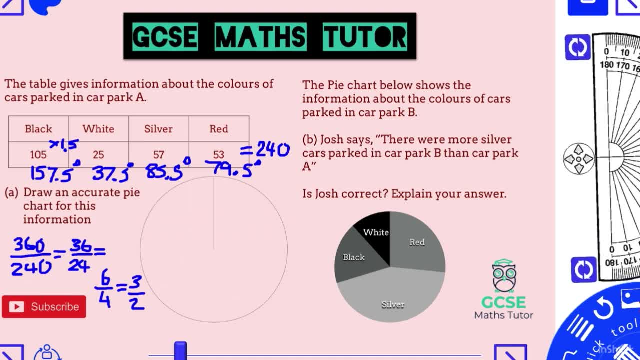 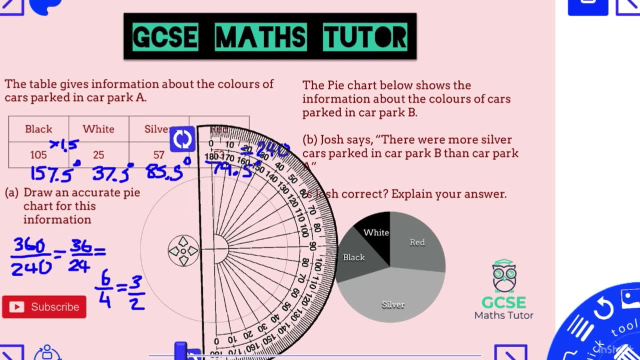 accurate. so it's best that we just try and draw this as accurately as possible, so if we just go for it and see how accurate we can make it again. this is quite a tricky one, because the pie chart is quite small on my screen so I could fit it all on for you, but let me try and do it as accurately. 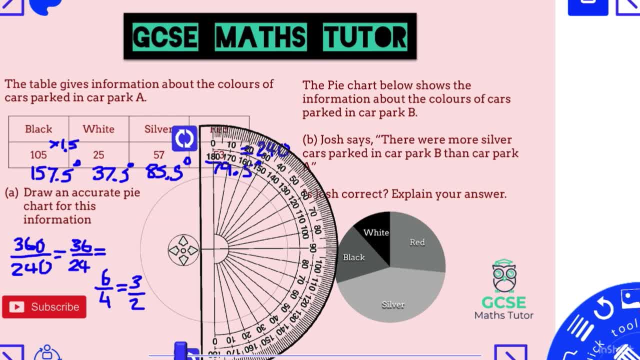 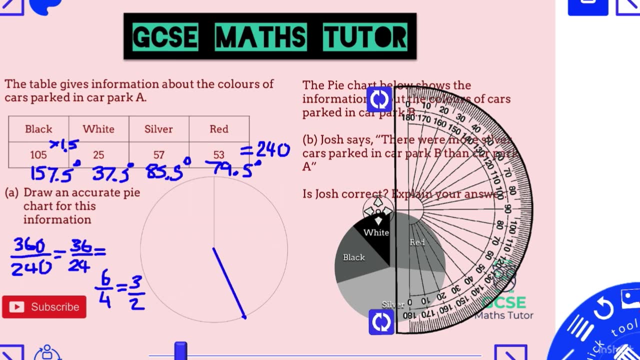 as I can. so the 157.5 is all the way down and off my screen a little bit. so let's see if I can. 155, 7.5 is around about there, okay, so if I draw that straight line in, there's 157.5 and then I'll. 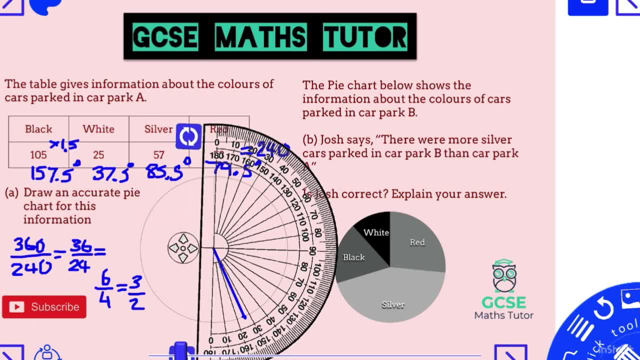 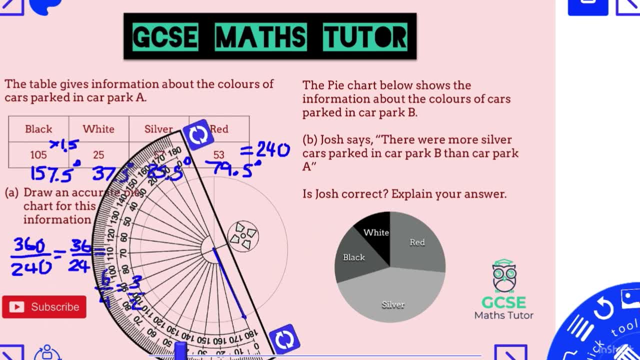 bring it back. let's twist it round and we've got 37.5 to go from that new one. there we go. very tricky when there's a lot on the screen. 37.5 is here, so that's quite a small one. there we go, just. 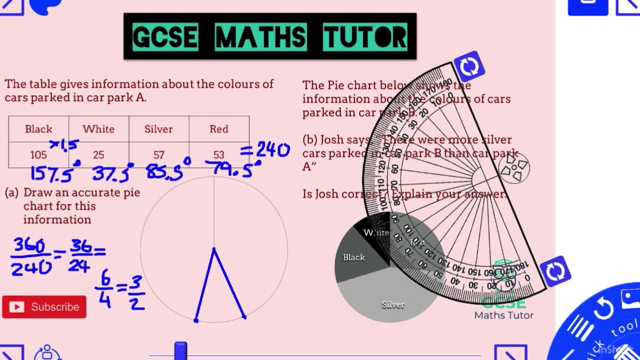 between 37.5 and 37.5 is here, so that's quite a small one. there we go just between 37.5 and 37.5 is here, so that's quite a small one. there we go just between the 137 and 138, and that is there, and then bringing it back on. 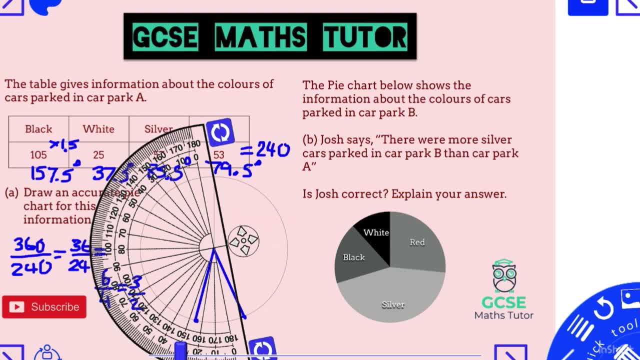 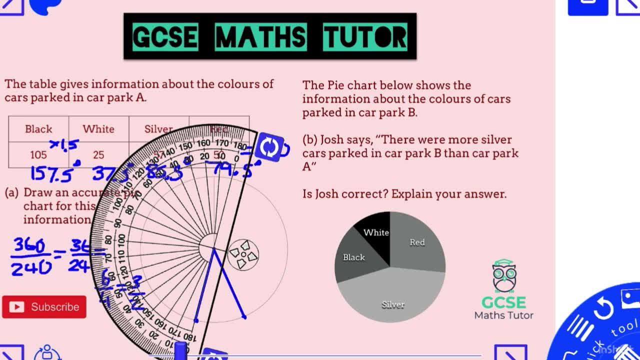 now what's the next angle? 85.5, okay, just about line that up. always got to make it as perfect as you can, so 85.5 goes up to. let's have a look. 85.5, just between those two. just about fit that in and join that up. 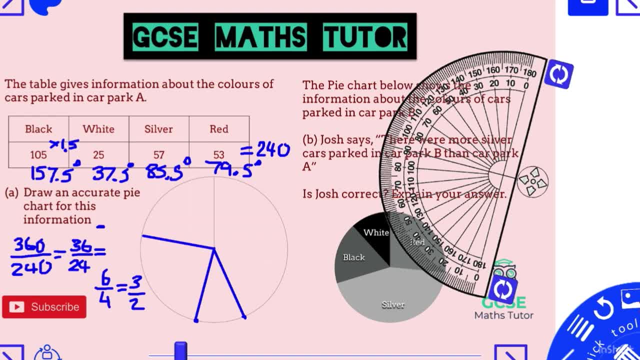 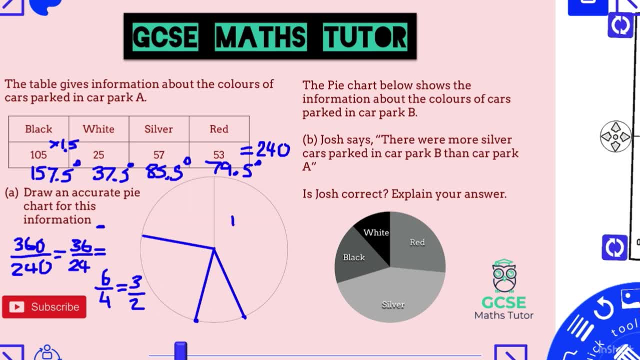 and then, thankfully, the last one's done for us, okay. so there, right, not the easiest of ones to draw that one, but let's put these pieces in. so we have black here, which was 157.5 degrees- I'm probably not gonna be able to fit these all in white, which was 37.5 degrees, just about fit. 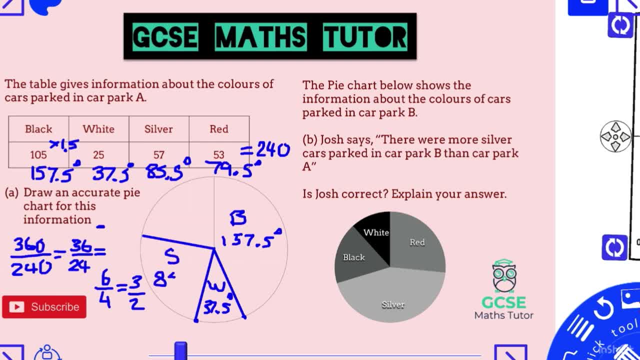 that in we've got silver, which was 85.5 degrees, and then we've got silver, which was 85.5 degrees, and then the last one there, which was red, which was 79.5 degrees. there we go now just as a little point here. that is probably a much harder one than you would have to do, obviously, without a calculator. 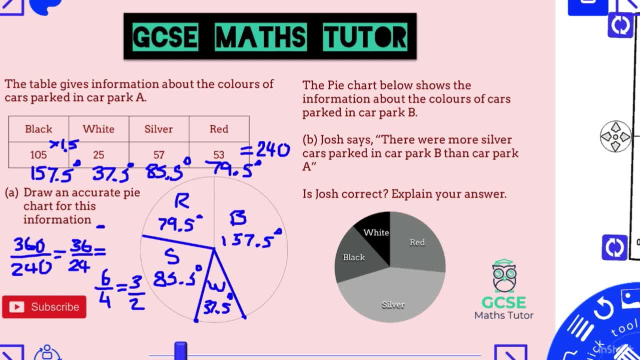 it'd be much more likely if it was a non calculator question, that they would all be even numbers, so they wouldn't get these point fives. but I just want to highlight to you that this could happen. you could get a point five in there and you know it's nothing to be worried about if that does. 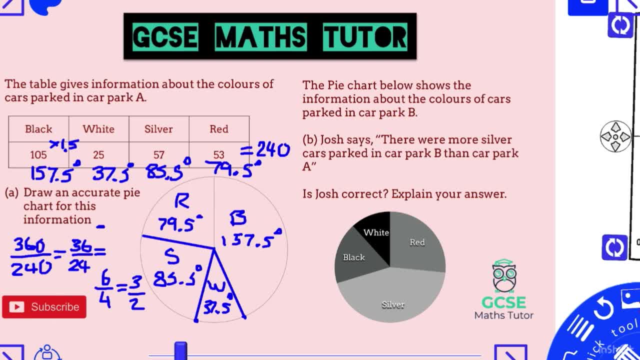 happen. you just try and draw that in and you'll get a point five in there and you know it's nothing to be worried about. if that does happen, you just try and draw it as accurately as you can. but, as I said, much more likely that you are going to get one. 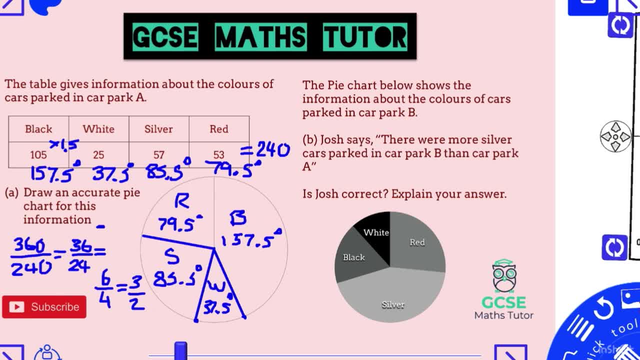 that has nice whole numbers in there. but there we go. that pie chart is drawn now onto this part b. it says there were more silver cars parked in car park b than car park a, where you can see. obviously the silver section is only 85.5 degrees in our pie chart and on this pie chart the silver 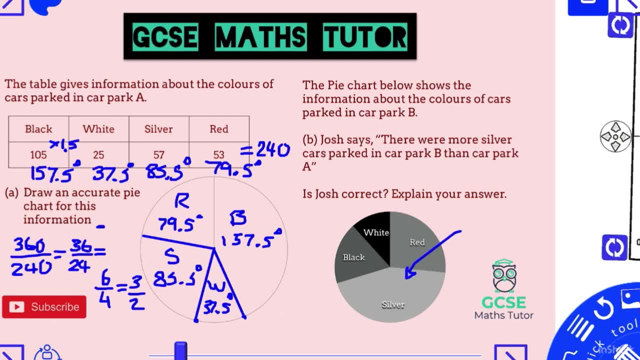 section is obviously quite large. it's almost half the amount. so logically you would say, yeah, there's more silver cars parked in car park b, but there's more silver cars parked in car park b, but there's. but in terms of this question, the answer is no. Josh is not correct if we think about our car park. 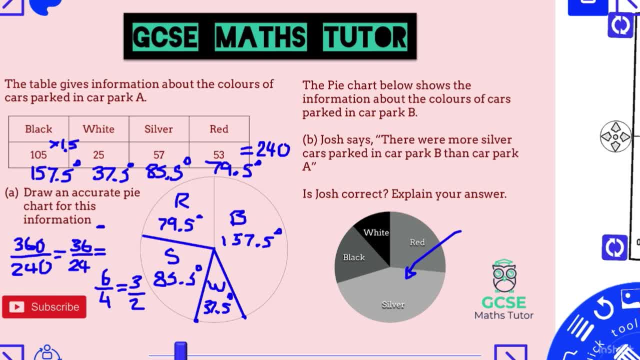 which had 240 cars in well, out of those, 57 were silver. now, if this car park here that is shown in the second one, maybe there's only 20 cars parked in that car park, and if there was only 20 cars- as an example, let's just imagine that there's only 20 cars here- then just less than. 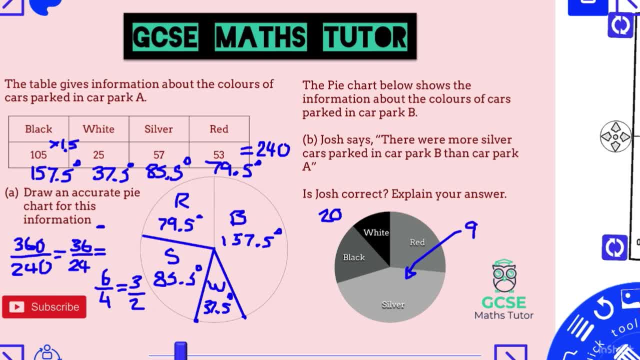 half. I don't know, maybe silver would only be nine cars. so nine cars in comparison to our 57 cars is clearly not as many, is it? so we don't know unless we know the amount of numbers. that seems strange saying it like that. unless we know the actual numbers behind the pie chart, then we can't make. 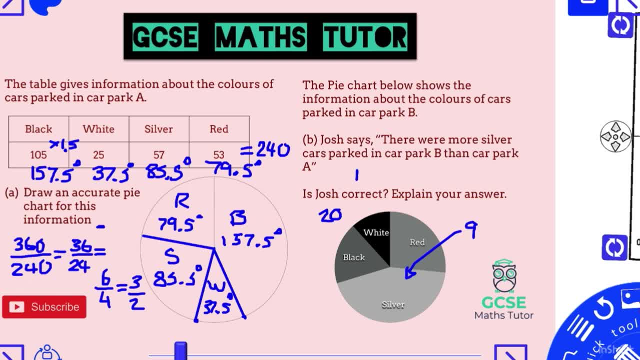 any comparisons, so we would have to say no, Josh is not correct, because we don't know any of the numbers behind the pie chart. we don't know how many cars are actually parts in there, so we can't make an exact. we can't make a comparison. a pie chart only shows proportion. okay, so it doesn't.